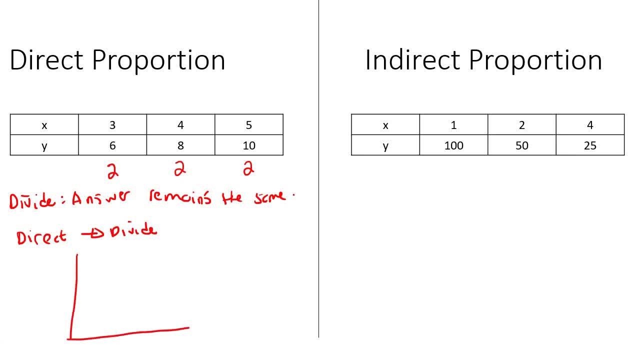 Perfect Now if we had to quickly go and draw this graph. I just want to show you what happens. So let's say we put x at the bottom and y at the top. So if, for example, you put x as 3 and y as: 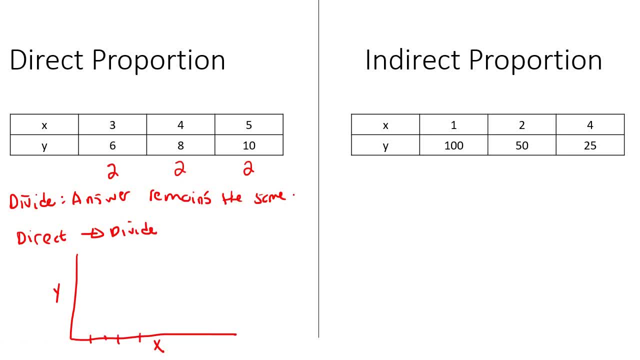 8,. so let's just put here 1, 2,, 3,, 4,, 5,, 6,, 7,, 8,, 9,, 10.. And then let's just put 1,, 2,, 3,, 4,, 5,, 6,. 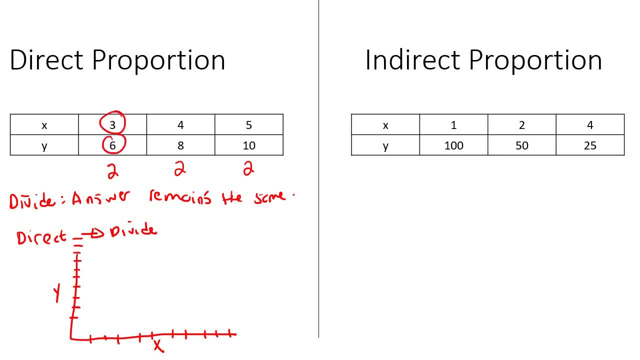 7,, 8,, 9,, 10.. So if you go put x as 3 and y as 6, so x is 3 and y is 6, that would be somewhere over here: 1, 2, 3, 4, 5, 6.. Yeah, so x is 3 and y is 6 over there. Now, if you had to go look at this: 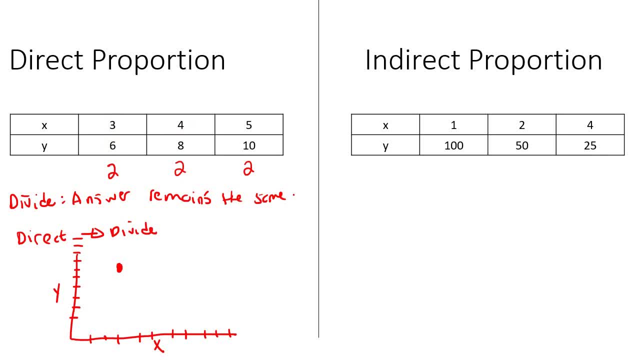 point when x is 4, y is 8.. So when x is 4, y is 8, that would be somewhere over there. So if you, and then when x is 5,, 1,, 2,, 3,, 4,, 5,, y is 10, which would be somewhere over there. So when you 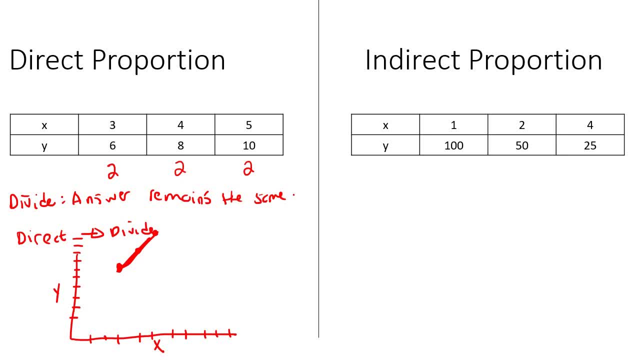 connect it, you would see that it's a straight line. Now, if you had to go- the way that it works is if you had to go back. I haven't drawn this perfectly, but it will actually always go right to the beginning. So I want you to know that when you have direct, it makes a straight line. So 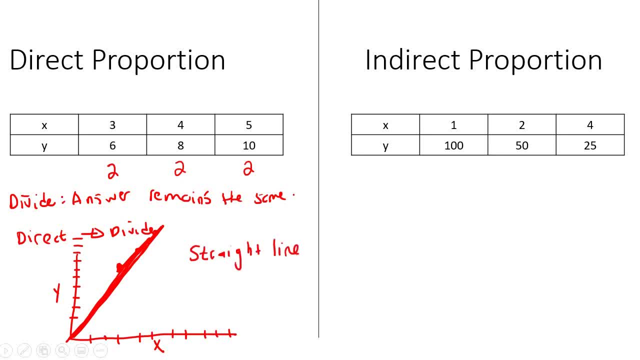 let's just say that it makes a straight line. Now let's look at indirect proportions. So if you had to go multiply these, that will give you 100.. If you had to multiply these, that will give you 100.. And if you had to multiply these? 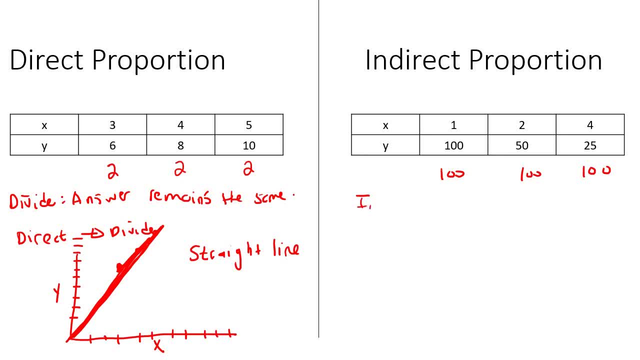 that would give you 100.. Ah, so when you are busy with indirect, the numbers will multiply. You must multiply, okay. Oh, but something I forgot to tell you about this one. Can you see that? what's happening to these numbers? Are they going up or are they going down? 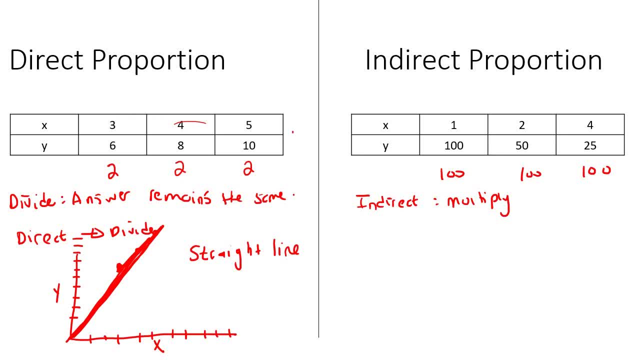 They are going up. 3 goes to 4, goes to 5.. So the numbers are going up. And look at what these numbers are doing: 6 goes to 8, goes to 10.. So what are these numbers doing? They're also going. 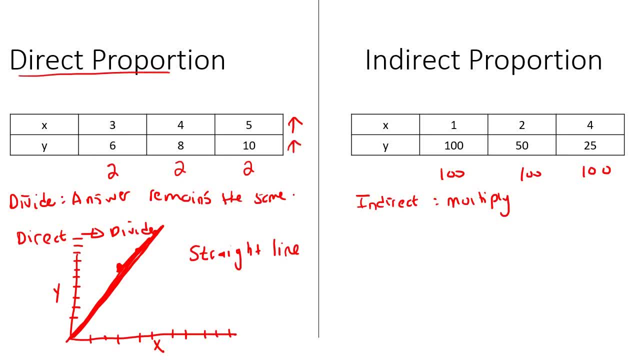 up. So that is what direct variation- direct proportion, sorry- does: When the one goes up, the other one goes down, And then if the other one, if the one goes down, then the other one also goes down. Okay, So that's something you need to remember. When they either both go up, 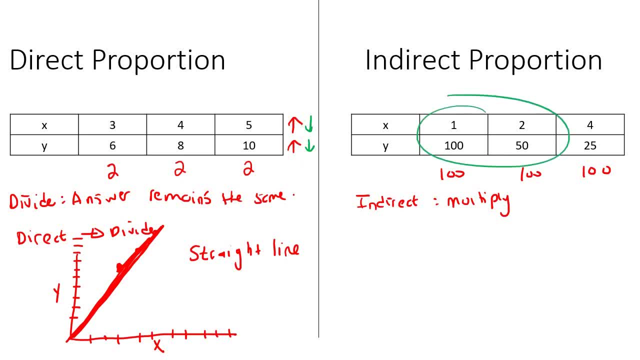 or they either both go down. But let's see what happens over here. Look what happens to these numbers. They are going up. So they're going up. But look at what happens to these numbers. They are going down. They're becoming smaller. 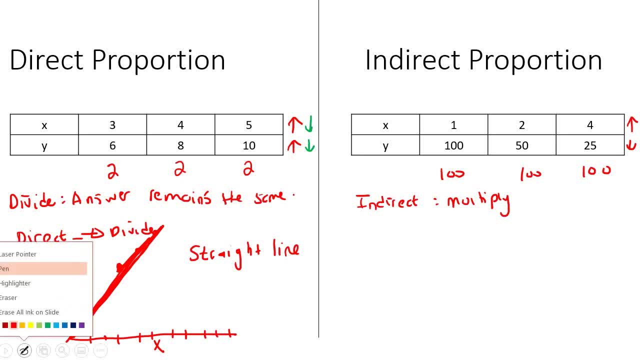 So when the one goes up, the other one is going down, And then, in some examples, when these ones go down, then the ones at the bottom go up. Okay, So here the one goes up and the one goes down With this one. if the one goes up, the other one goes up, And if the one goes down, 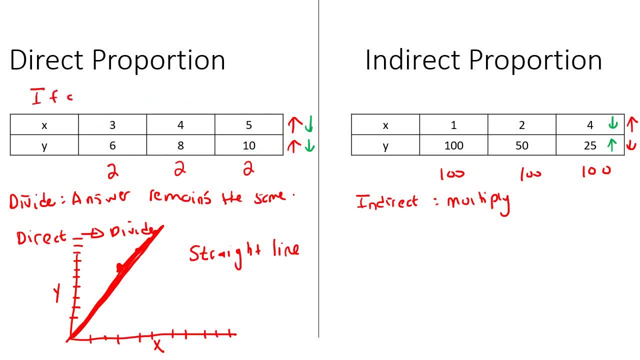 the other one goes down. So let's just say here, if one goes up, the other goes down. Here we can say: if one goes up, goes up as well, And then we can also say: if one goes down, the other goes down, And then with indirect proportion, if one goes. 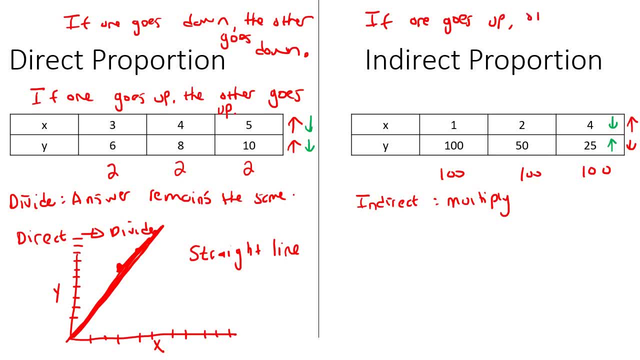 if one goes up, then the other one goes down, Other goes down, And if one goes goes down, then the other goes up. Okay now, if we're to just go draw a graph- x and y- now I'm not going to go draw 100 little lines, But if x is one, let's just 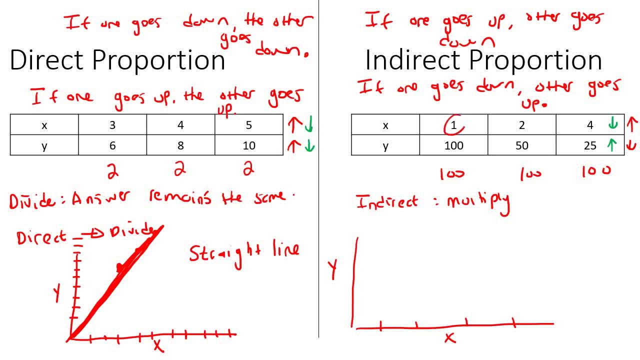 put 1234.. So if x is one, then y is a very big number, which is 100. So let's just put it up here, So that would be over there. If x is two, then y is 50. So that would be over. 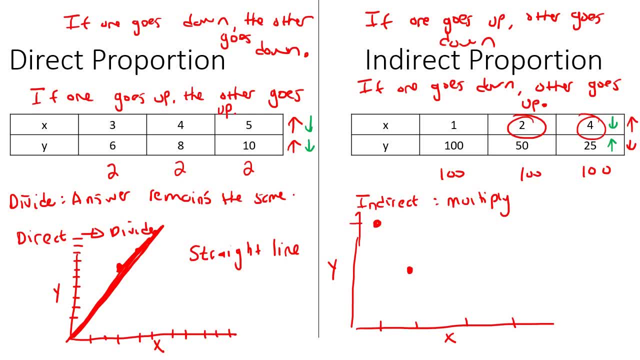 there, And if x is four, y is 25, which would be over there, And so it's not a straight line. you see that it actually makes a curve. it makes a curve, And so that's the summary you need to know. Now we're just going to. the most important part, to be honest, is this: 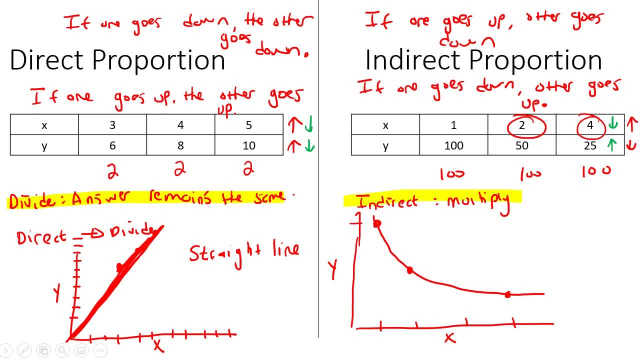 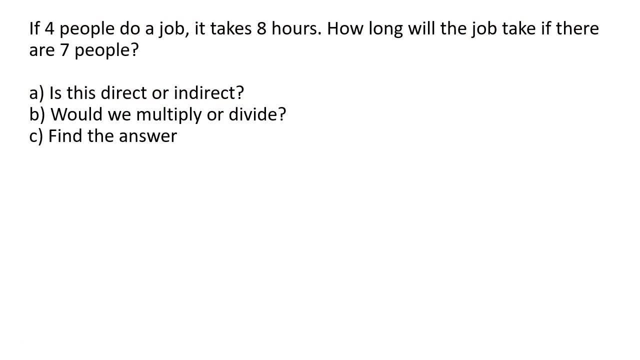 part here. this part is going to give you everything you need to know, So just remember that. Okay, now let's go do some examples. Okay so if four? so you got to think about these questions carefully. If four people do a job, it'll take eight hours. How long? 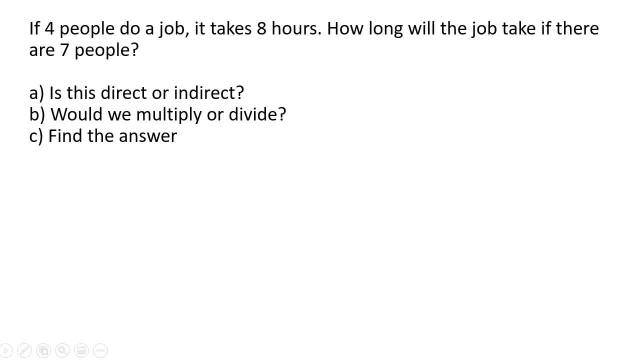 will the job take if there are seven people? Okay, so think about it. there are four people and they're busy doing a job. Maybe they are painting a room or building a house, And how long does it take? Eight hours. Now, all of a sudden, we are going to make more people. 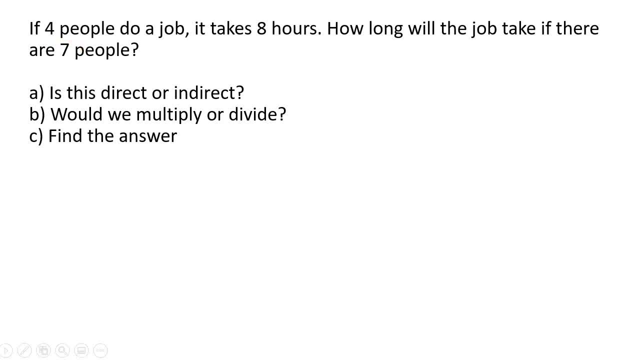 Okay. so what will that do to the job? Will it make the job take even longer, Or will it make the job go faster? It should make it go faster. So what are we doing to the number of people? the number of people are going up. What are we doing to the number? 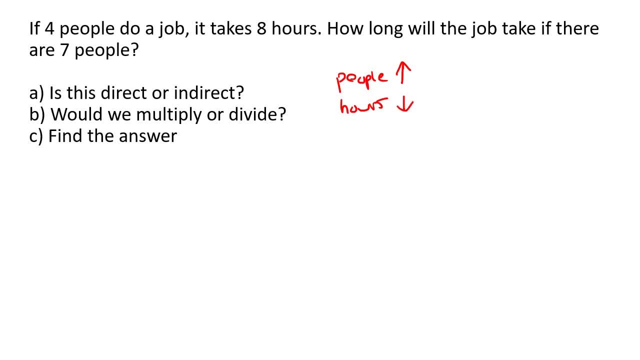 of hours. The number of hours is going to go down because it's going to go faster. So if it was eight hours, maybe now it's going to be five hours. So the number of people are going up, but the number of hours are going down. So if you remember from the previous slide, that's 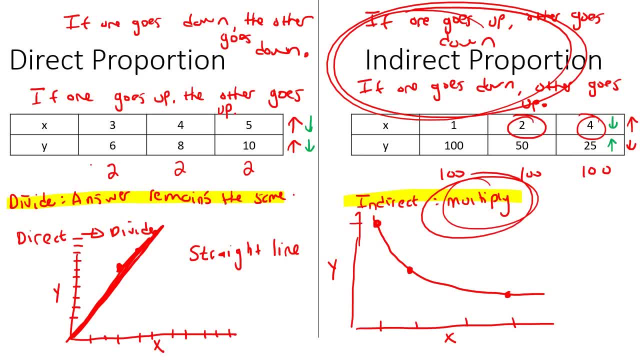 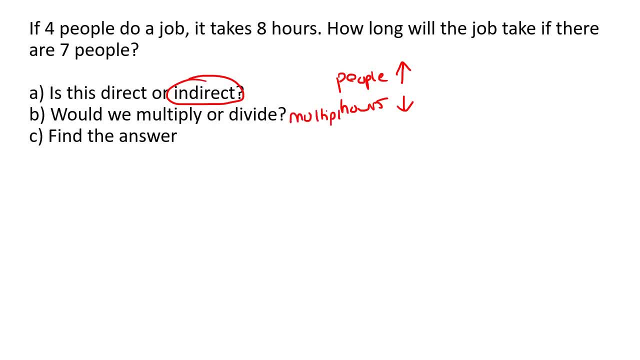 going to be indirect proportion, And so multiplying is what we want to do. So this is going to be indirect, Okay, so should we multiply or divide? we should multiply, And now we're going to find the answer. So all that you do is the following: there's people and there's 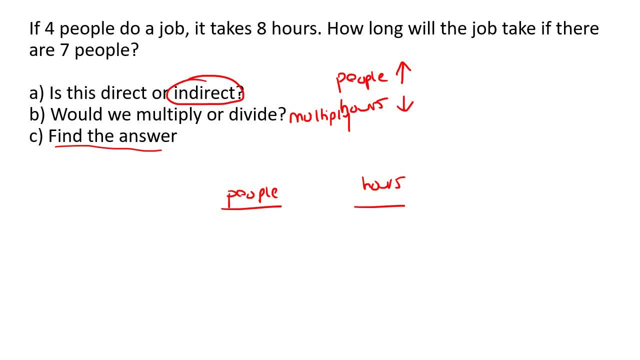 hours. Okay, so now we're going to find the answer. So all that you do is the following: there's four people and there's eight hours, And then you're just going to say four people and that goes with eight hours, and then seven people goes with this many hours. Okay, Now. 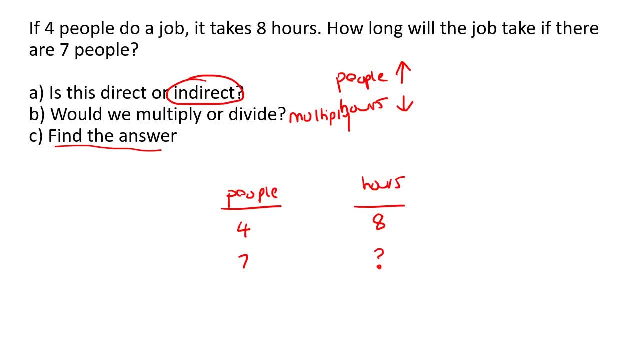 we're not going to do any multiplying across. like I've showed you in previous lessons, that is not something we do with direct indirect. What we do here is we said we should multiply, So we multiply. now you might be confused: should we multiply these numbers Or should? 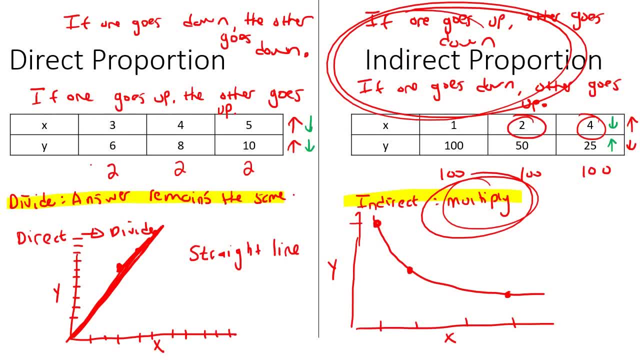 we multiply these numbers, Or because let me show you here: you see, x could have been maybe people, and then y could be hours, for example, and so. so, as we just said, um, one of them is like people and one of them is like hours, and so it's these numbers that we. 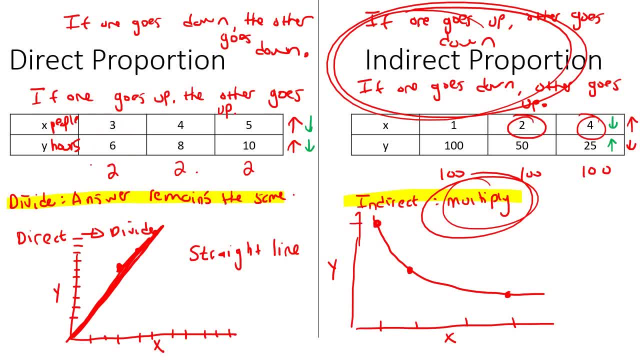 multiplied, okay, or divided, it's not. um, you don't go this way, okay. so it's going to be the different categories, like people and hours. you either multiply or divide those. so we said for this question: we are going to multiply, so here's people and hours. you're going to multiply those two. 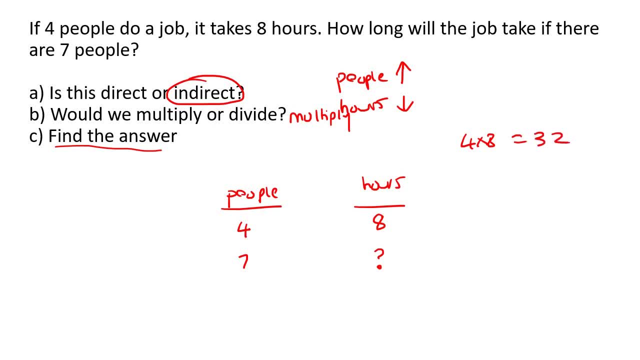 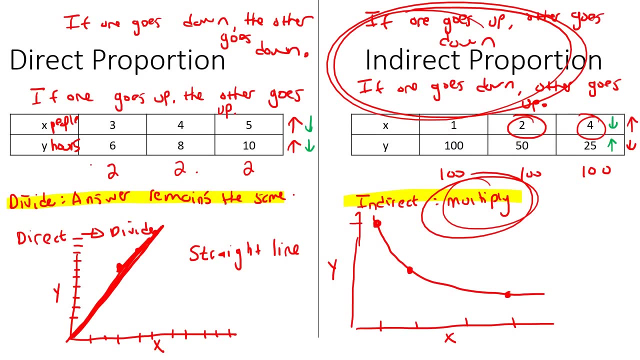 so 4 times 8 is 32, and then if you multiply these two so we can call this x, then that must also be 32. okay and so because remember, we said that when you multiply the numbers, they must always give you the same value. so when we multiplied these two, it gave us 32. so when you multiply those, 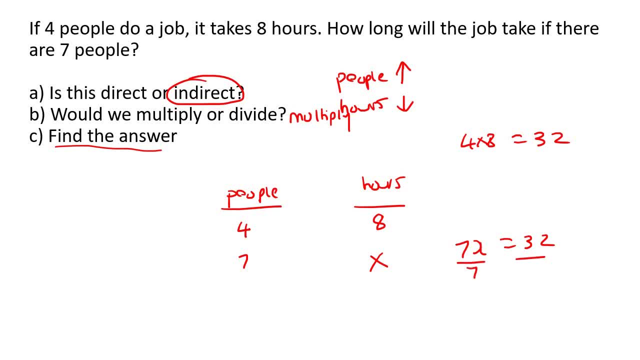 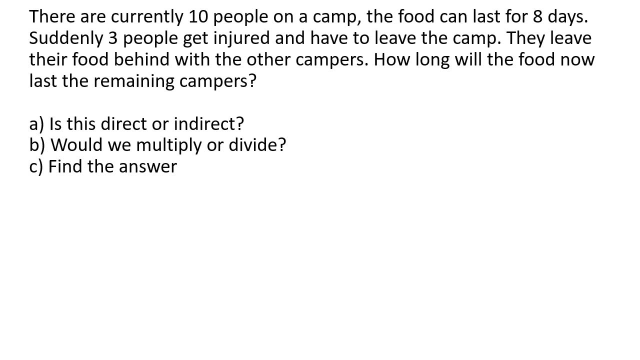 two, it will give you 7x, and then to get x alone, you divide both sides by 7, and so x will be 4.57, and then that'll be measured in hours. there are currently 10 people on a camp, okay, so you must picture that when you read these. 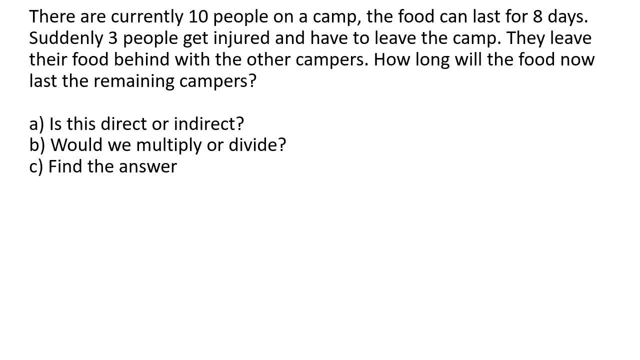 questions. there's 10 people. they're having a camp. the food can last for eight days, so the food that they have can last them for eight days. okay, suddenly three people get injured and they have to leave the camp. they leave their food behind with the other campers, okay. so how long will the 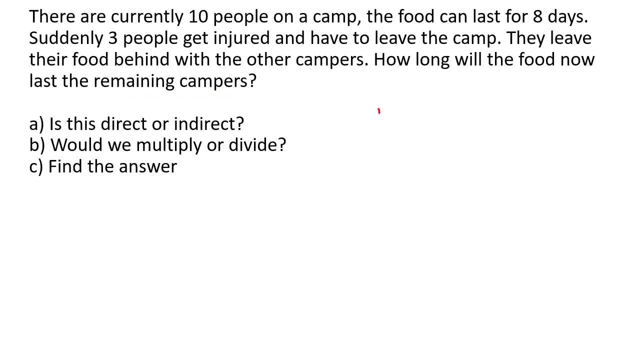 food now last the remaining people? okay, so think about that carefully. there were 10 campers and all together, the food would last for eight days. okay, so the for the, the food would last for eight days. now, all of a sudden, three people have to leave the camp. okay, so that means there are. 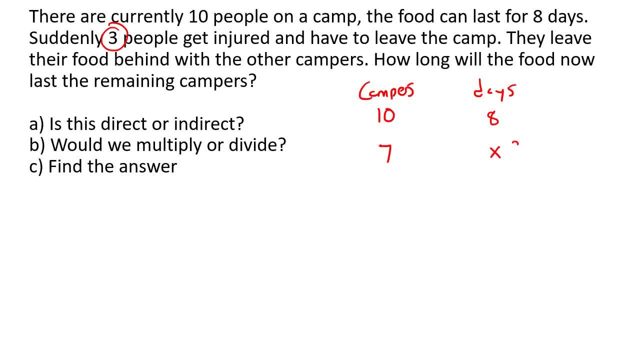 seven campers left over, and you need to try work out how many observers will be left over and if they're, who then Recap? how many days will the food still be available? Now you've got to think about it carefully. What have we done to the number of campers? 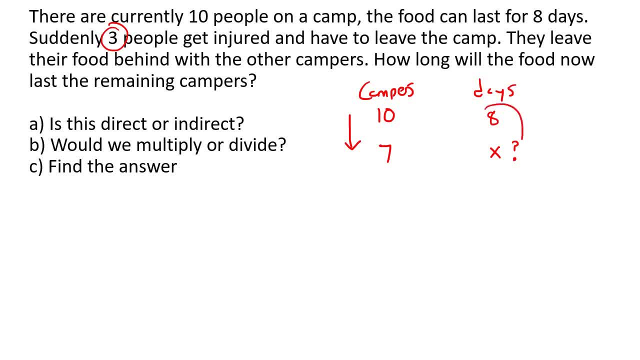 We've made the number of campers go down. Now you've got to think about this. Imagine you are together with a bunch of people, so there's 10 of you all together and there's eight days' worth of food for all of the 10 people. okay, 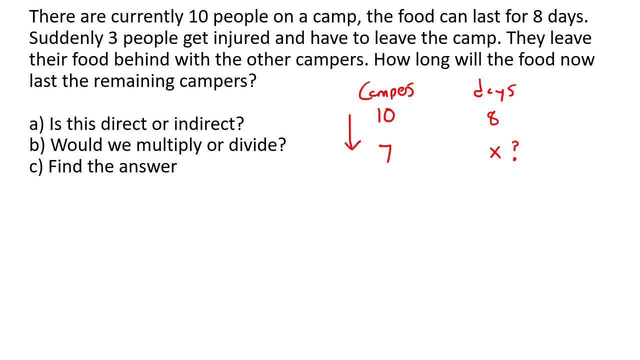 Now three of the campers have to leave. So that remaining food, is it going to last you guys longer now, or less time? It should last you longer, So the amount of days should go up. So you see, the number of campers is going down. 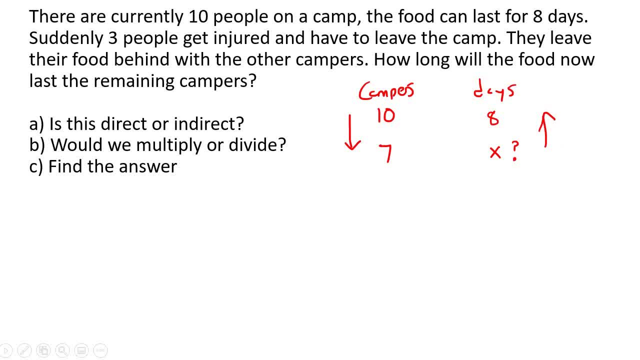 but the number of days that the food will last is going up because now there's less people to eat the food so it will last them longer. So when the one is going down, the other is going up. That is called indirect, okay. 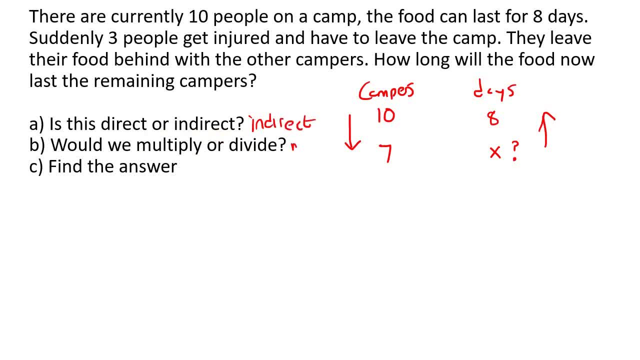 So should we multiply or divide? Well, we've learned that with indirect you must multiply. And now it says: find the answer. Okay, so you're going to multiply these two numbers together, which is 80.. And then, if you multiply these two, that must also give you 80. 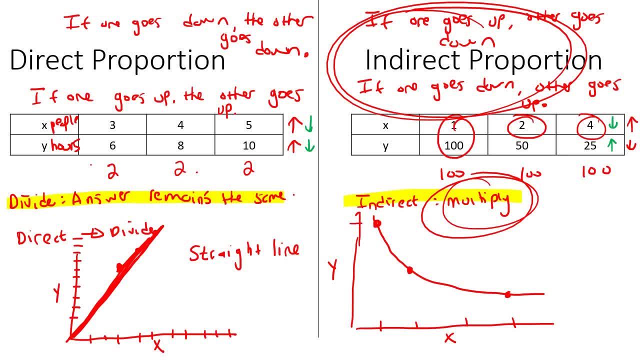 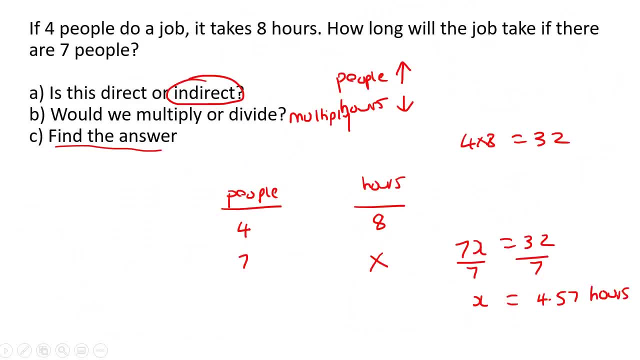 Because remember, with indirect, when you multiply, it should always stay the same. So in this example it was 100,, 100, and 100. So it must always stay the same. So now, if you want to get x by itself. 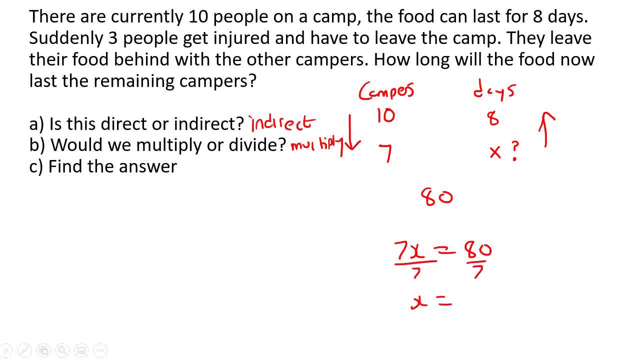 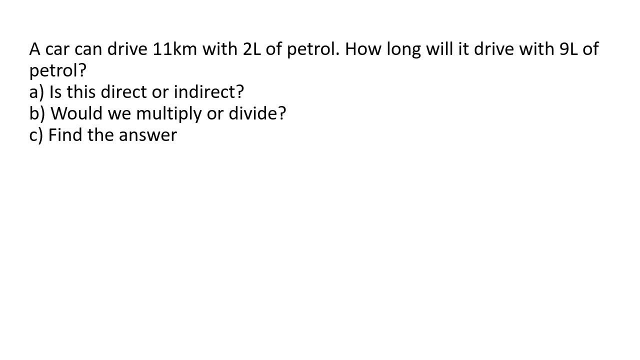 you have to divide both sides By 7,, and so x would be 11.43 days. So now that there's only 7 campers left, the food will last for 11.43 days. A car can drive 11 kilometers with 2 liters of petrol. 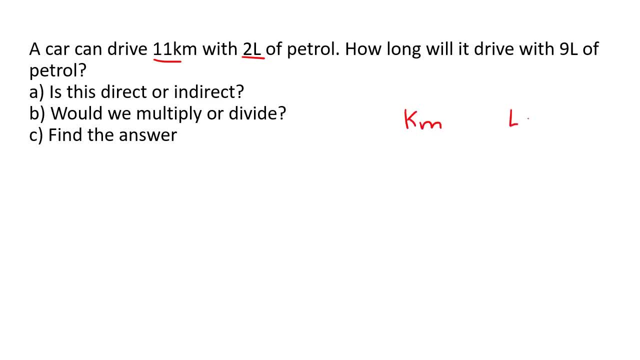 Okay, so we've got kilometers and liters of petrol. Okay, So here we have 11 kilometers and 2 liters of petrol. Now it says how long will it drive with 9 liters of petrol? Okay, so the amount of petrol, they are increasing it. 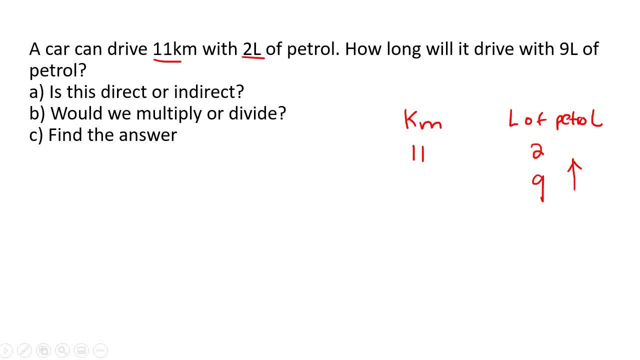 Can you see that From 2 to 9, they are increasing the number. Now, if you know the way a car works and if you just think about it carefully, a car can drive 11 kilometers with 2 liters of petrol. 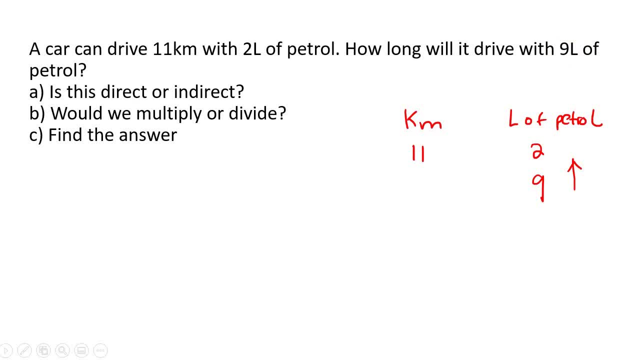 How long will it drive with 9 liters of petrol? So if you have more petrol in the car, it can drive further. So the number of kilometers should also go up. So because, Because both of them are going up, or if both of them are going down, or if both of them are going up. 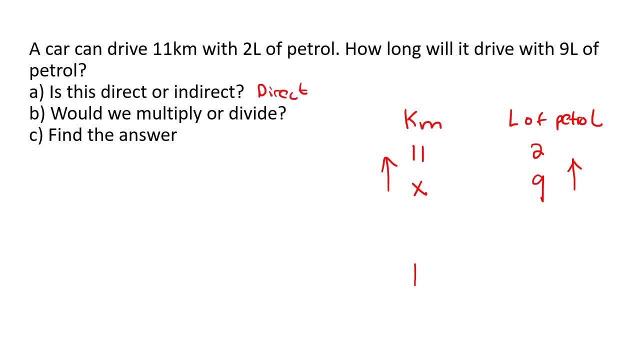 that is called direct. If one of them is going up and one of them is going down, then it's called indirect. Okay, Or if one of them is going down and the other one is going up, that's also called indirect. But if both of them are going up or if both of them are going down, 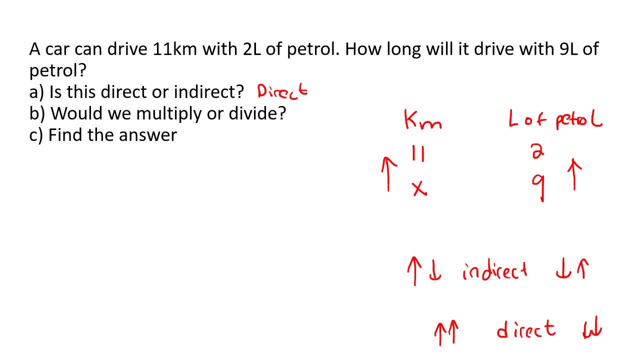 then it's called direct. Okay, So because it's direct, we are actually going to divide. So you can take, for example, I always like to choose the bigger number first. So you could say 11 divided by 2.. So we could say 11 divided by 2, which is 4, point whoopsie, which. 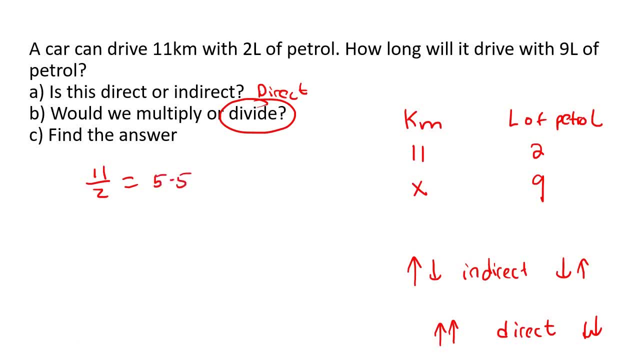 is 5.5. Okay, And then you can, and then you must divide these two as well. So x divided by 9 must also be 5.5. Because when you divide them, the number must stay the same, just like we. 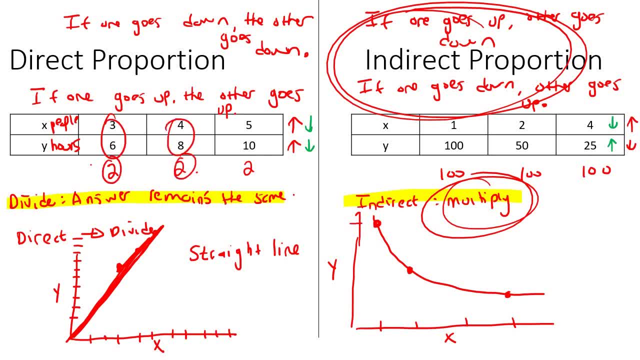 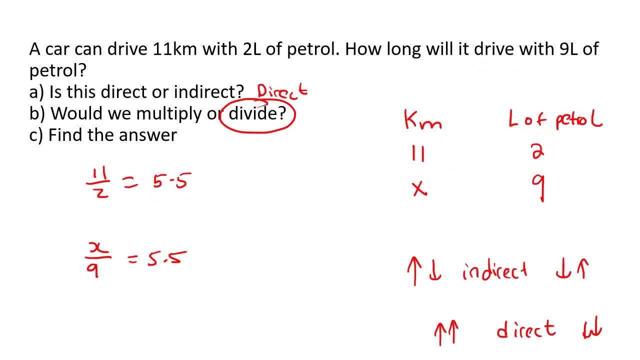 learned over here: When we divided, we got 2.. When we divided, we got 2.. When we divided, we got 2.. So here we divided and we got 5.5.. And I said this one divided by this one. So now, 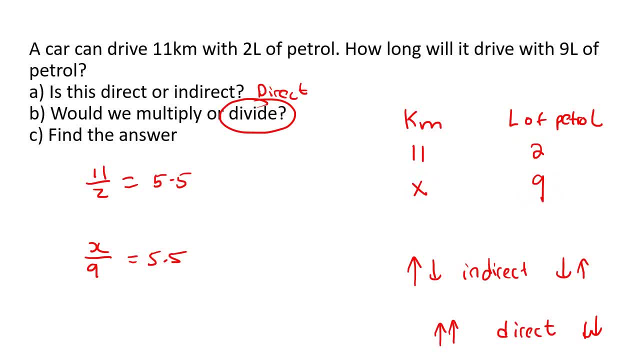 we're going to say this one divided by this one, and that must give us 5.5.. Now the way to get this: 9 by itself. this is where you need to understand equations. So, if you remember the chapter with equations, this is a divide sign. So the opposite of that is a multiply. So you're going to multiply. 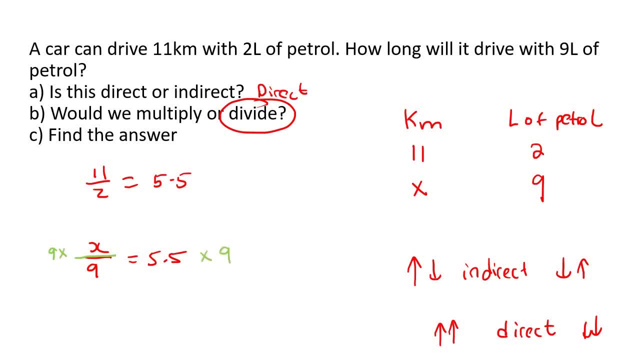 this side by 9.. And what you do to the one side, you do to the other side, so that these nines would cancel over here, And so you end up with x equals to 5.5 multiplied by 9.. And so x will be. 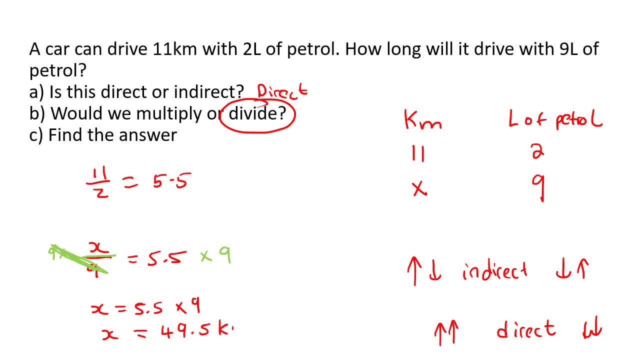 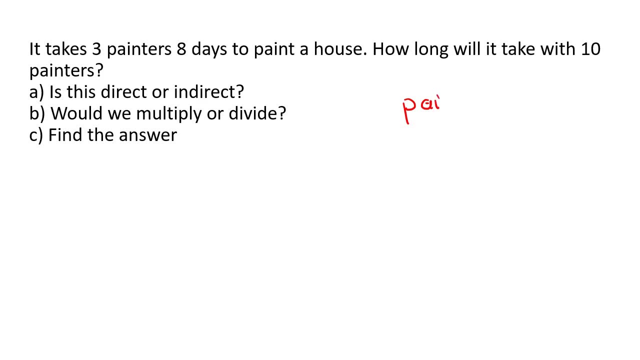 49.5 kilometers. Okay, so you see how the car can drive further because it has more petrol. Four more examples. This one says it takes three painters. Okay, so we've got painters And we've got days. So we've got three painters and eight days. Now. 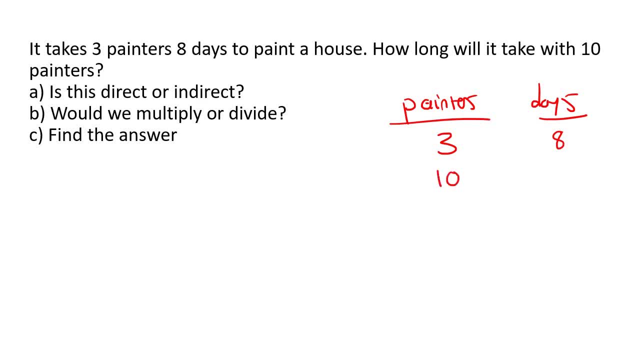 how long will it take with 10 painters? So we're going to say 10 painters over here. So now let's see what they did to the number of painters. Well, what did they do? They increased the number of painters. So you've got to think about this carefully: If there are three people painting, 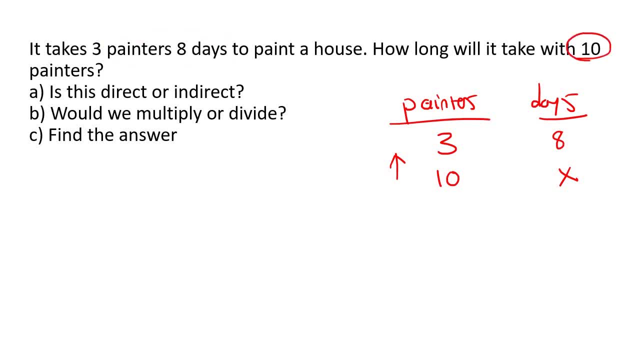 a house, it takes them eight days. Now if you have 10 painters, it should go even faster. So instead of it being eight days, it'll become less. So this number is going to go down. So these numbers increased and these numbers decreased. So that is called indirect. That means 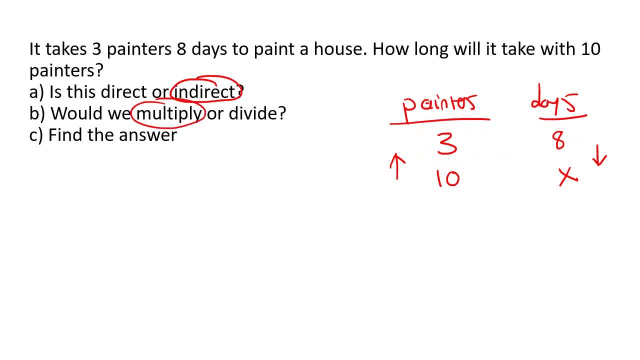 we will multiply. So we're going to multiply these two numbers together, which is 24.. And we're going to multiply these two numbers, which is 10x. And we know that when you multiply the values must be the same. So we can say that 10x will be equal to 24.. And so to get x by itself, you divide by 10,. 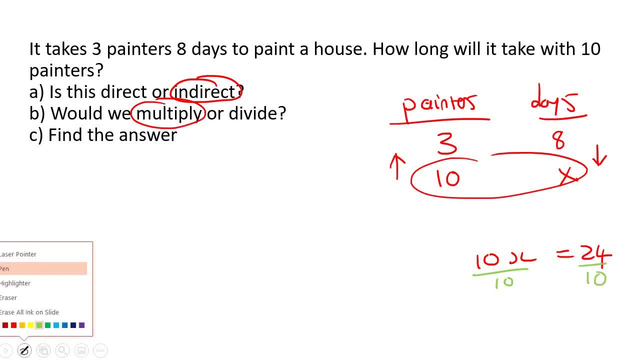 and then what you do to the one side, you do to the other side, And so x will be. so if you cancel that out, x will be 2.4 hours. This one says that John can run 10 kilometers in three hours. Okay, 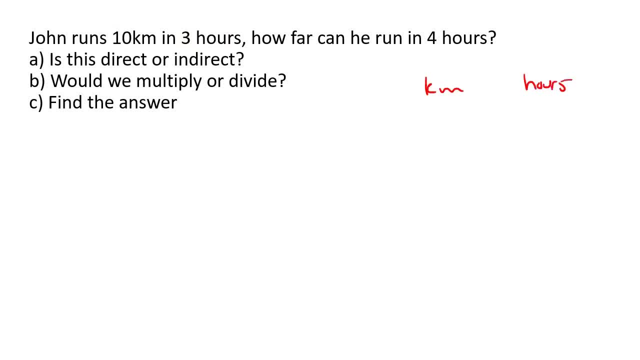 so it's the kilometers and hours. Those are the two different categories. So John can run 10 kilometers in three hours. How far can he run in Four hours? Okay, so the number of hours. you see how they changed it from three to four hours. So that's the number of hours, And then 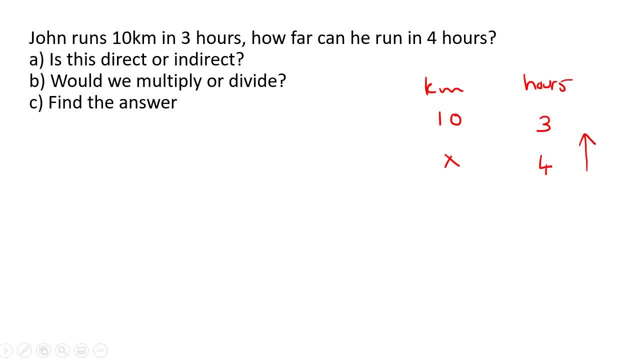 the number of hours. you see how they changed it from three to four, So they increased that. So I show it as an increase like that. Now you got to try to think about this. So John can run. picture this in real life: In three hours John runs 10 kilometers. Okay. so if he can run for four hours, 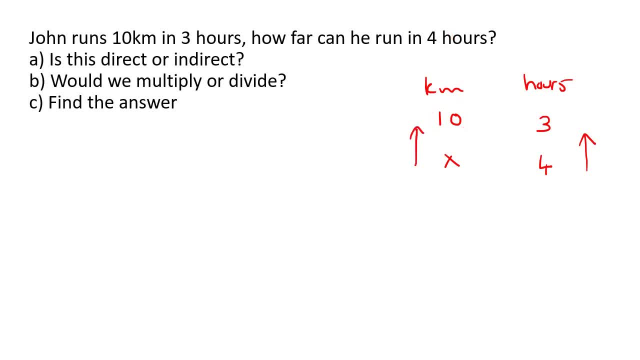 he should be able to run even further. So this number should go up as well. So you see that both of the numbers are going to go up. So when they're both going in the same direction, that is called direct, where you divide. So we're going to always like to take the big number. So we're going to say: 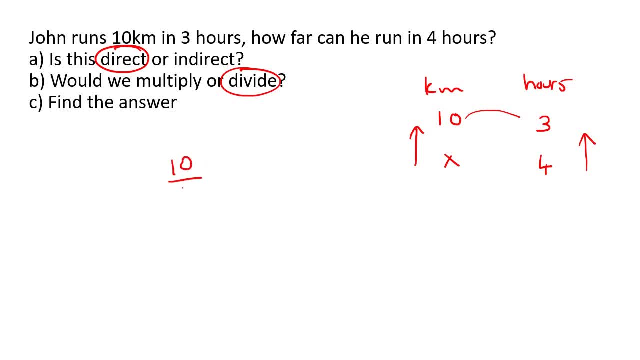 10 divided by three. Or let's say 10 divided by three. And then here you're going to say x divided by four. And we know that these two must be equal to each other Because we learned in the very beginning that 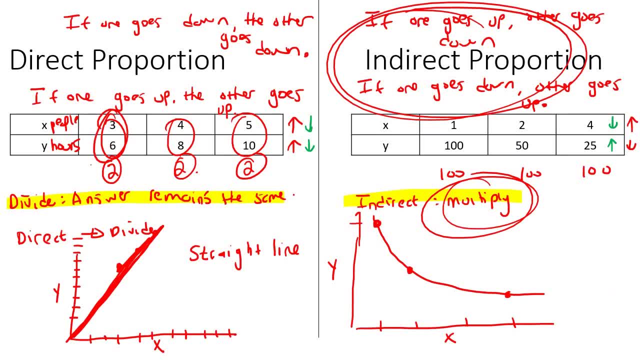 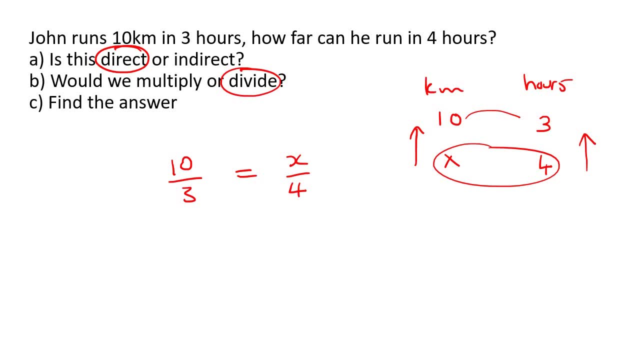 when it's direct, then when you divide, the answers must always be. the answers must always be the same. Okay, so we divided them and then we make them equal, And so the way that you do this now is you need to get rid of this four. Now you see that this four is going to be the same, So 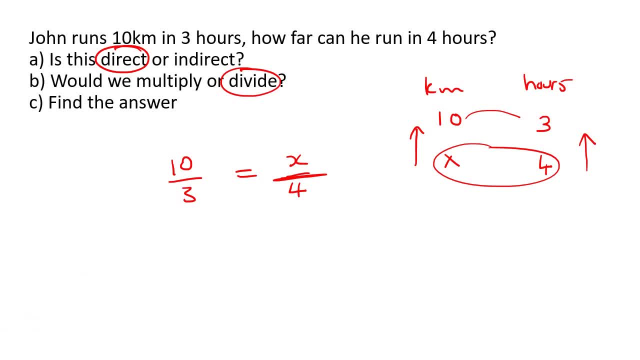 you can see that the four is at the bottom. That is means that these two are being divided. So the opposite of divide is multiply. So what you do to the one side you must do to the other side. So these fours are going to cancel. And so you end up with x equals 13.33.. And that would be measured. 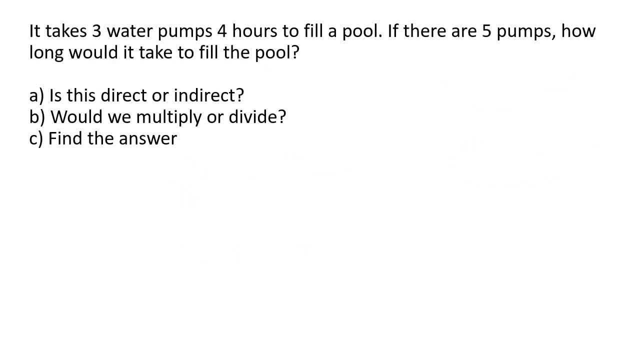 in kilometers. Two more examples: Well done, if you've made it this far, That's awesome. So here it says that it takes three water pumps Four hours to fill a swimming pool. So let's say, you have like a swimming pool, for example. 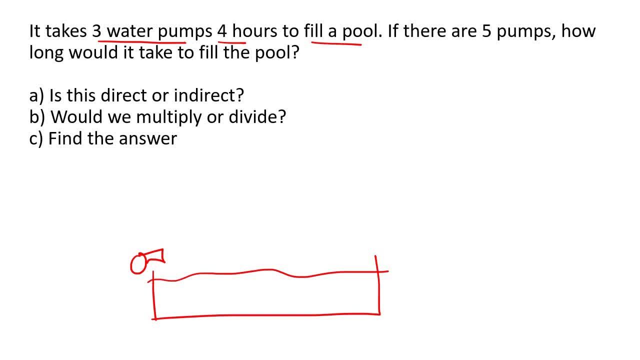 And you've got these water pumps. Now, let's say, we draw a little pump like that And that pump is spraying water into the pool, Okay, And they said that we have three of those. Now, if you have three of those, it says that it will take four hours to fill the pool. Now, 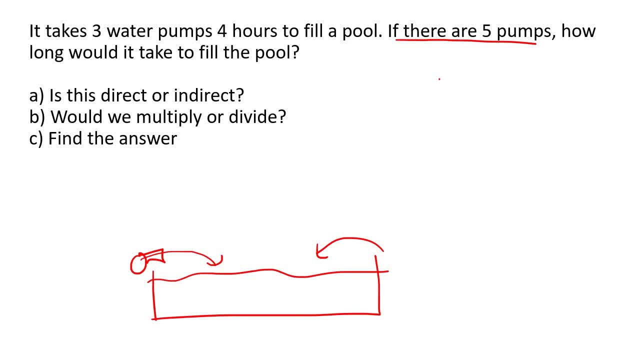 what if there are five pumps? Ah, okay, So the different categories here is going to be number of pumps and the number of hours. So when they have three water pumps, then it takes four hours, And if it is five water pumps then we. 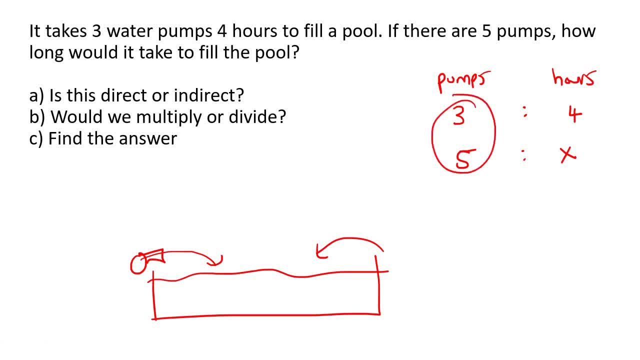 need to figure out the number of hours. So what are they doing to the number of pumps? Well, they increased it from three to five, So they increased it. So I'll show that with an up arrow. Now you got to think about this carefully. They're adding more water pumps now, So does that mean it's going? 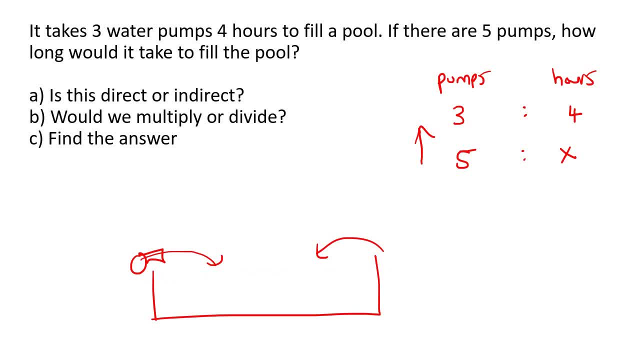 to be quick, faster to fill up the swimming pool, Or is it going to take less time? It's going to take less time. So this number is actually going to go down. So it's going to take less time. So this number is actually going to go down. Some learners, they want to say up because it's going to go faster. But when something goes faster, it means that the time will become lower. Okay, so you see, the number of pumps is going up, but the number of hours is going to go down. That is called indirect, And so we multiply. So I'm going to multiply these two values. I'm going to multiply these two values. I'm going to make them equal. Okay, And so now we need to get x by itself, And so we divide both sides by five. 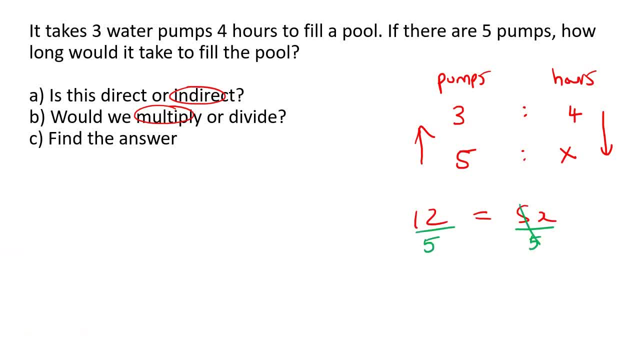 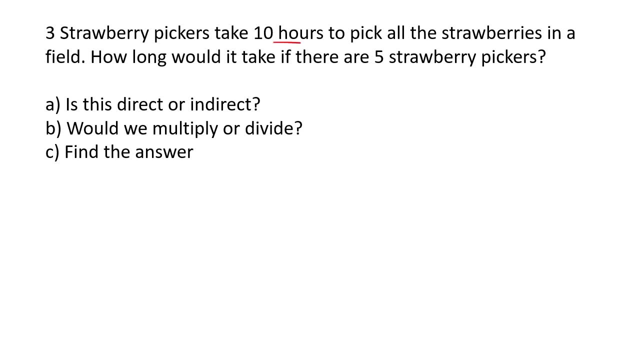 So that this cancels. And so you end up with x equals to 12 over five, which is 2.4 hours. Here's our last example: Three strawberry pickers take 10 hours to pick all of the strawberries in a field. How long will it take? Well, let's first put our category So. 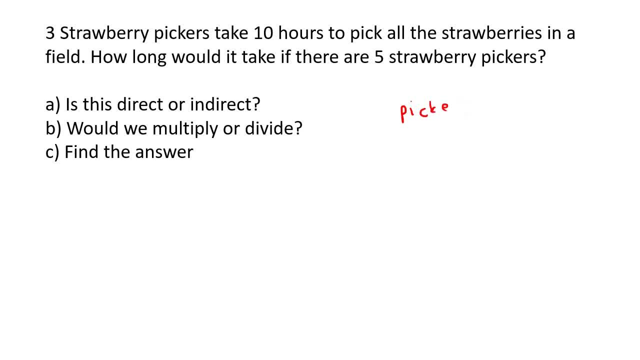 the number of pickers and the number of hours. So if you have three strawberry pickers, it'll take 10 hours. Now, if you have five strawberry pickers, how many hours would it take? So the number of pickers is increasing from three to five. So we